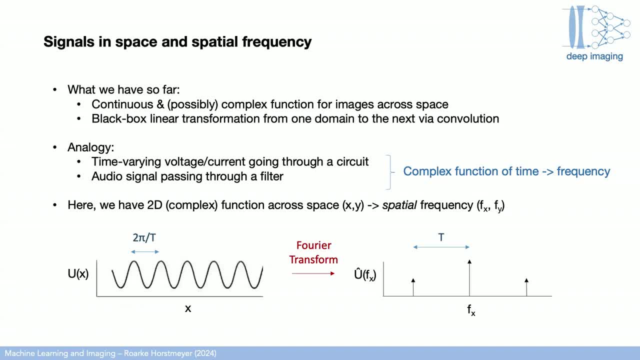 So when I draw 1D functions across space it might not make too much sense, So just bear with me for a second. But we have some function right. u of x Here I'm drawing it as a sinusoidal type function. 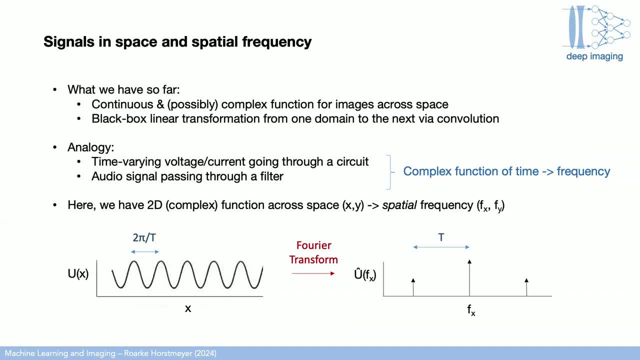 It has some periodicity, t right how often those oscillations occur across a distance? You can measure the distance, Because this is a function of x space, And the Fourier transform of this- hopefully this isn't too surprising- is going to produce three delta functions. 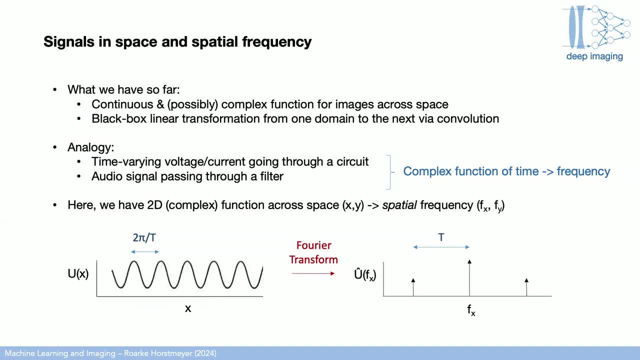 The first delta function is going to be the DC offset right, Because this function is not centered around 0. So you just get a constant term And then the other two define the periodicity of this sinusoid And so that distance from the delta function to this either. 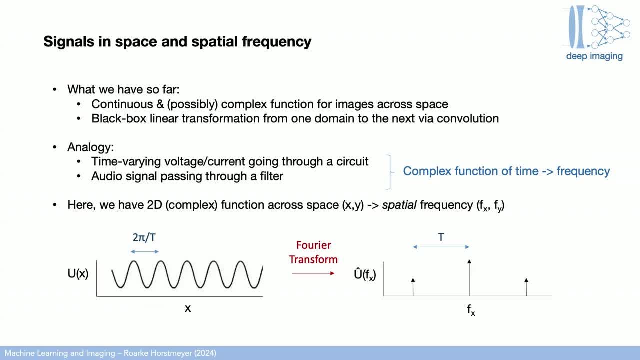 one of these peaks right that are defining this side lobe of this three-pointed Fourier transform is going to be equal to the periodicity t. OK, so that's kind of abstract, But really what we're talking about are two-dimensional functions. 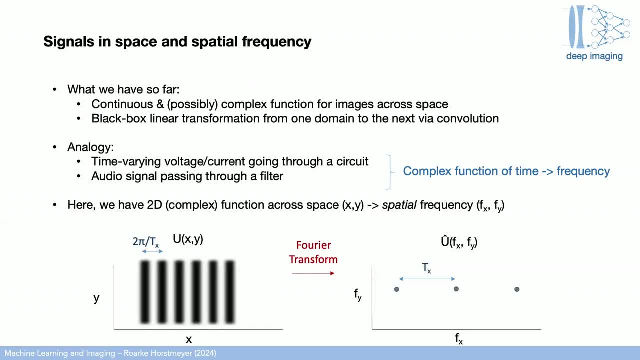 And so really, what I mean is picture some painting on the wall. there that's a bunch of stripes, And those stripes happen to be vertically oriented And they kind of aren't just perfect black white, black white, They kind of roll off. 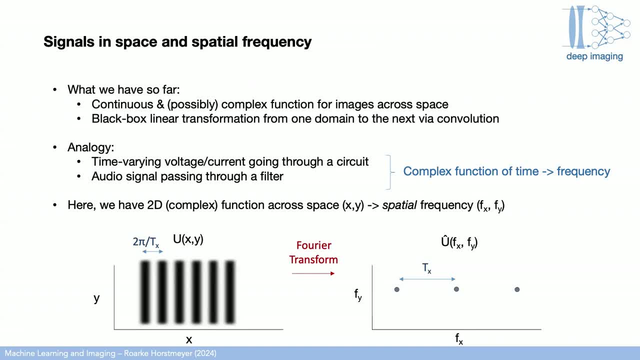 They go black to gray, to white, back to black. So they're kind of shaped stripes- right, I don't know the right term- Faded stripes. The fading happens to follow a sinusoidal distribution: the gray level Right, Where again black is being close to 0. 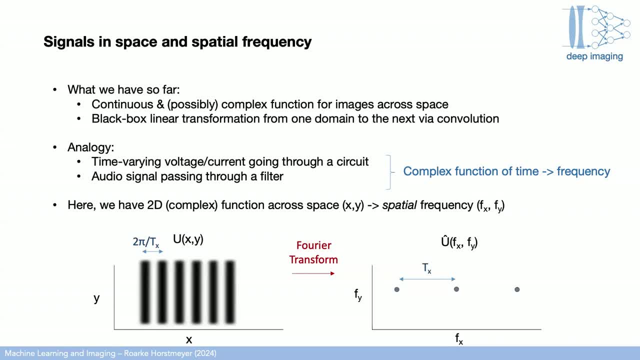 in our quantitative description of that stripe, because 0 means there's no light coming from it And white is close to 1, or close to whatever max value we're interested in, because that means the most light is coming from those white areas. 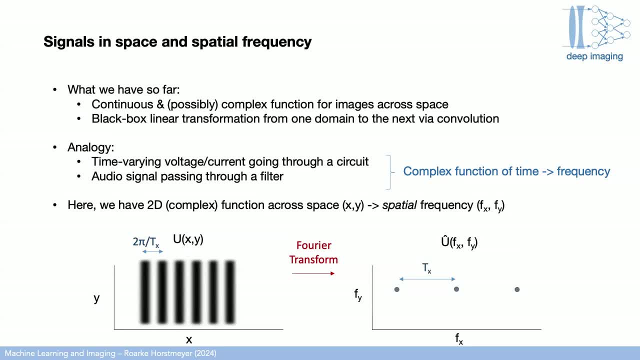 in our picture, And so we're going to be taking Fourier transforms of those two-dimensional pictures, right, And so, as I'll get into, Fourier, transforms are easily extended to any number of dimensions, And so you can think of a two-dimensional Fourier. 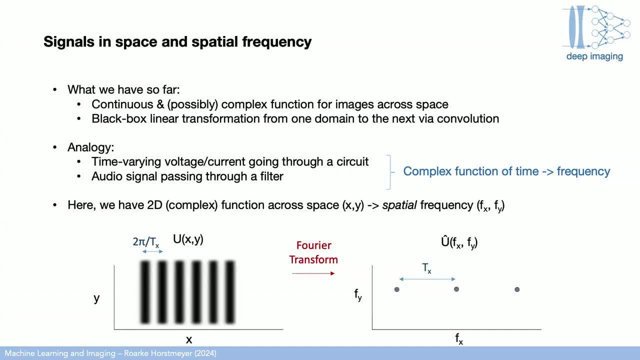 transform as some transform of that. that's kind of similar to the one-dimensional Fourier transform. If you did a two-dimensional Fourier transform of that stripe pattern, you would end up with a function, a two-dimensional function, where you get three dots. Again, most of the function is 0 except for these three dots. 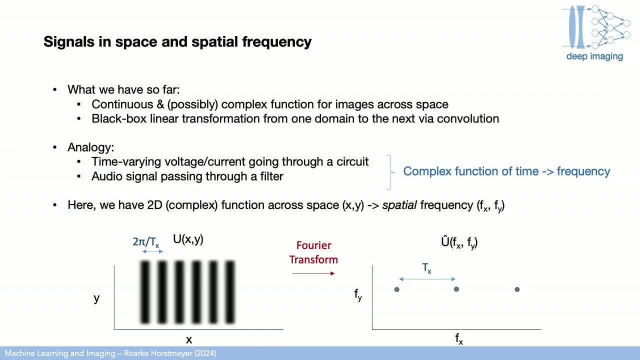 These three dots are like the delta functions I just pictured. Again, you can think of a two-dimensional Fourier transform as a two-dimensional Fourier transform. Again, their periodicity of the stripes on the wall are going to define how far apart those points are. 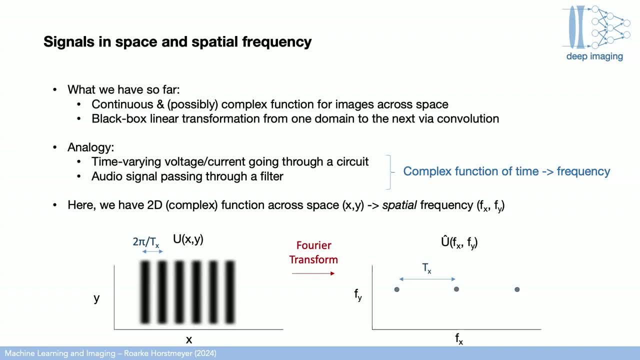 So if there's finer stripes, the periodicity is shorter And the distance, the frequency spacing, is larger right, And vice versa. Does that make sense? So it's the exact same thing, but we're just talking about it for two-dimensional functions. 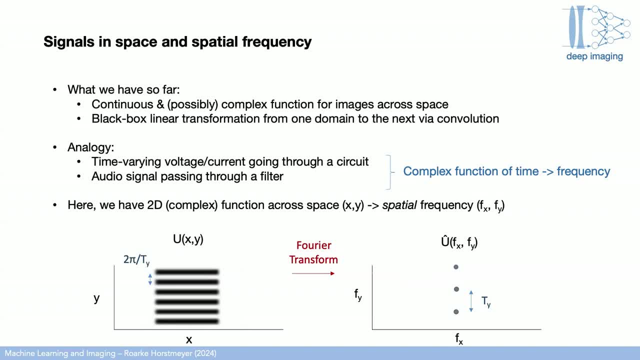 And so if I flip the stripes And drew horizontal stripes, had that as my input and I took a Fourier, 2D, Fourier transform of that, I would get vertically-oriented stripes- Sorry, vertically-oriented dots- in my Fourier transform, Because these points are saying yes there. 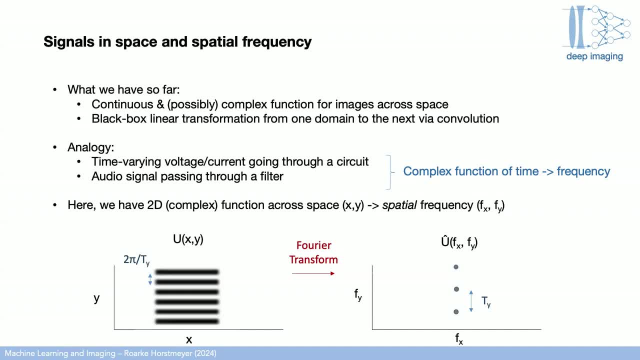 is energy at this frequency, spatial frequency offset, And nowhere else is there energy. There's no other contribution. There's no other contribution to the image that I can describe as stripes of different periods of speech, So I can just look at different periods. 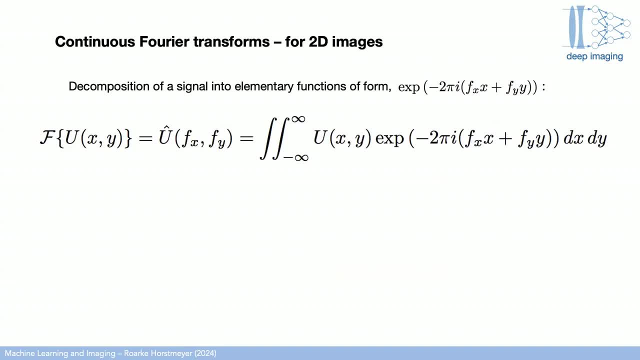 OK, And so this is the equation for this two-dimensional Fourier transform. It's the same as a one-dimensional Fourier transform, And here I'm using again continuous math and assuming complex functions. So use any complex function, pretty much. 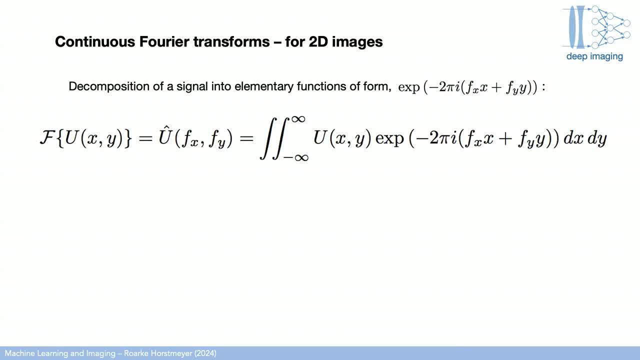 There's maybe a few limitations on you, But in general, for most scenarios of interest, an arbitrary, complex function, we can apply this type of transformation to it. It's a linear transformation. It takes the form of this integral equation in continuous space. 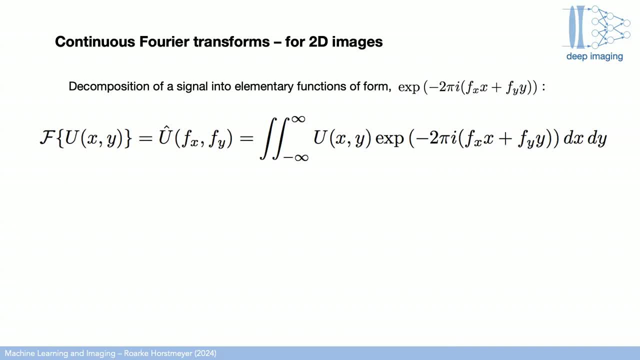 But generally we like to write these transformations out in shorthand And so whenever we write a Fourier transform out in shorthand, we'll use this F applied to the function OK, The function of interest or the quantity of interest, And also when we write Fourier transforms. 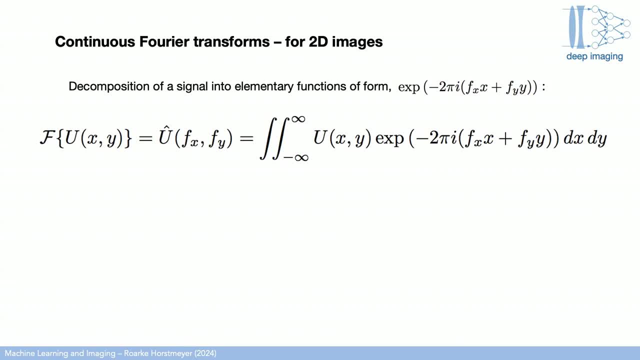 we'll put a little hat over the representation and frequency states. OK, It's the weighted sum of the input times. these are the stripes, different stripings, That's this complex exponential. Think of the complex exponential just in terms of a sine, let's say, or a cosine. 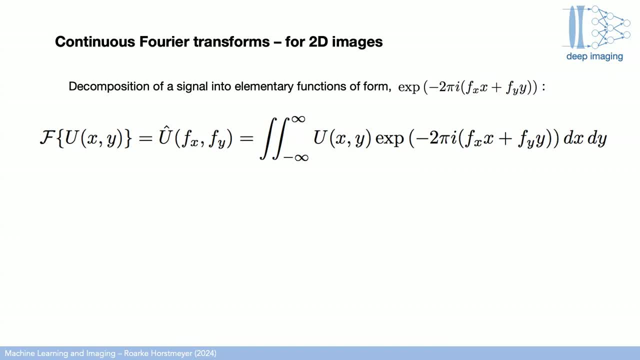 This is a bunch of cosines with different frequencies. After that, Here the frequencies are across space, So they're called spatial frequencies And they are literally different periodicities of striping. OK, It's the easiest way to think about it. 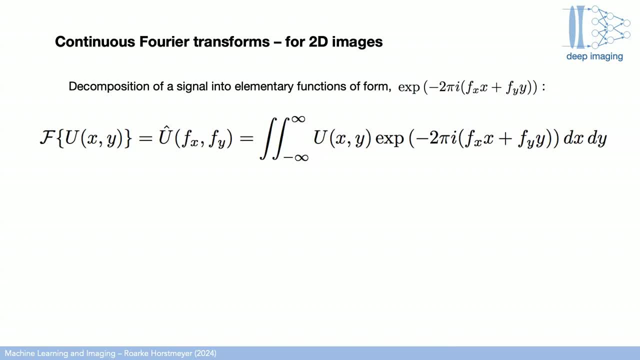 And so you have a picture And you said, hey, I want to describe that picture, decompose it into lots of stripes. Some are broad stripes, some are shallow stripes and they can be at any orientation. The sum of all those stripes, weighted sum. 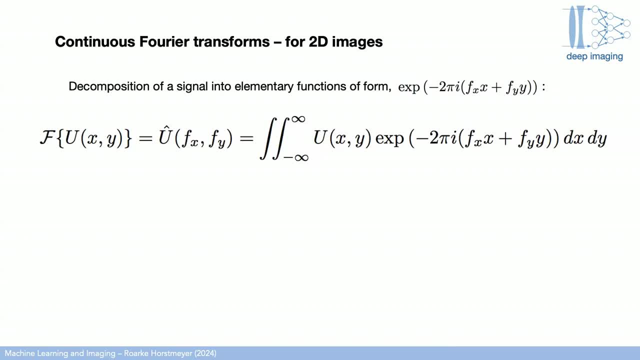 some could be positive, some could be negative- will give me my final picture. That's what this Fourier transform is, What distribution of stripe patterns describe the final picture of interest. OK, so any Fourier transform has an inverse Fourier transform, Or rather there is an inverse Fourier transform operation. 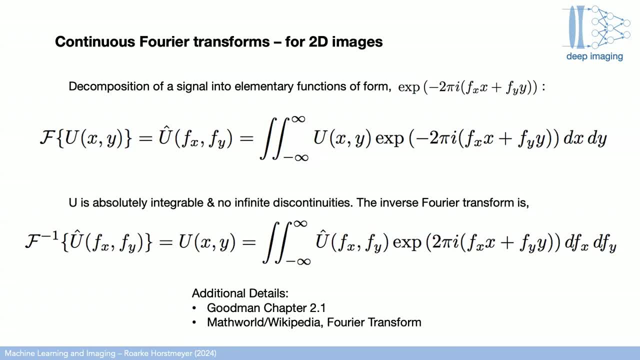 It's effectively the same thing, just flipped right. So you take a Fourier transform in the computer, You can just: it's a dot FFT2.. You can do an inverse Fourier transform: It's IFFT2.. And you'll recover exactly what you started with. 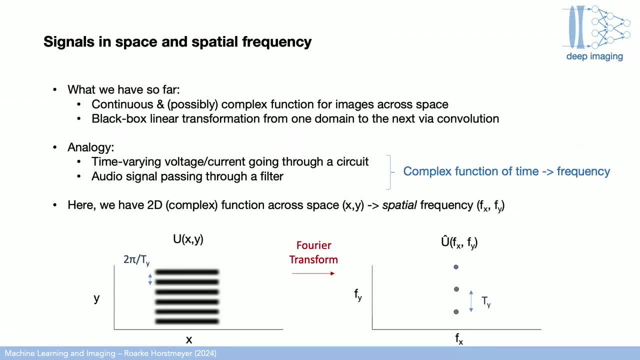 And so there's mappings from these points to those stripes, And that's pretty simple. This is saying: hey, Here's your input, There's a DC offset And then there's a frequency of interest that you should draw right across the whole space. 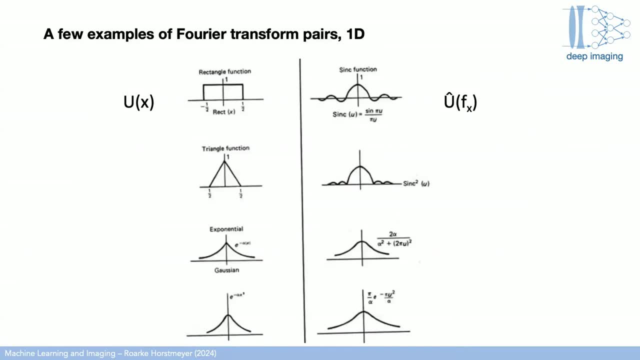 And so these are some common Fourier transforms that we'll encounter in this class, because we're going to- not surprisingly, we're doing lots of convolutions. As we'll get to, we'll do lots of Fourier transforms. They go hand in hand. 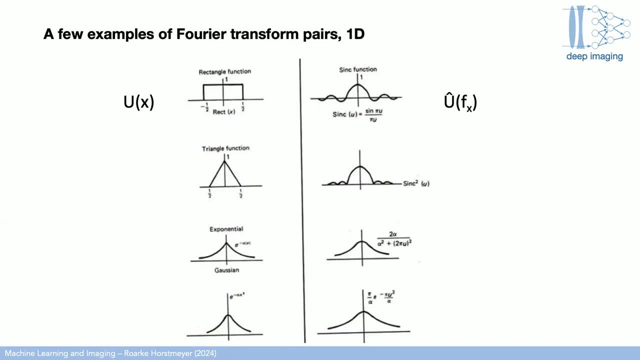 Remember that signal processing. So we have A rectangular function which is zero outside of some bounded area and one inside that bounded area. The Fourier transform of a rect function is a sinc function. The triangle becomes a sinc squared function. It's exponential becomes a Lorentzian function. 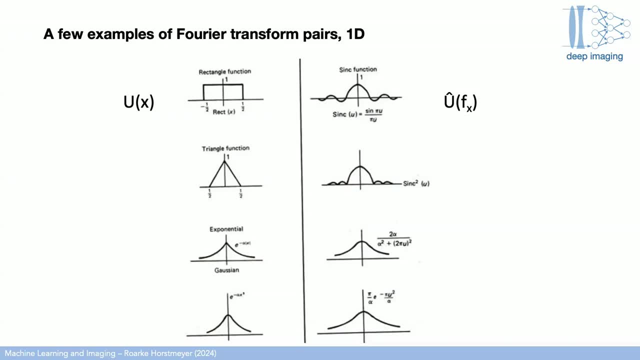 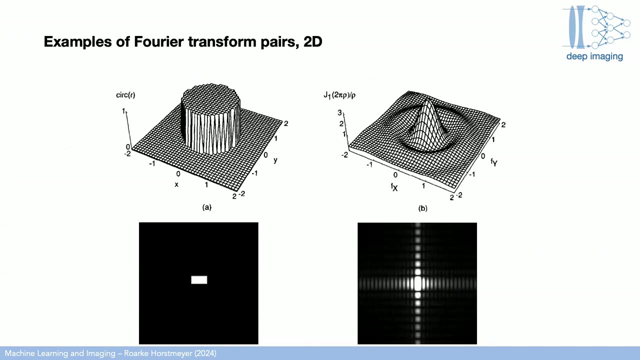 And then Gaussians have this nice property- weird property- that when you take a Fourier transform of a Gaussian it's still a Gaussian. That's kind of nice. So here are just some two-dimensional Fourier transforms. We have a circular function or a circ function. 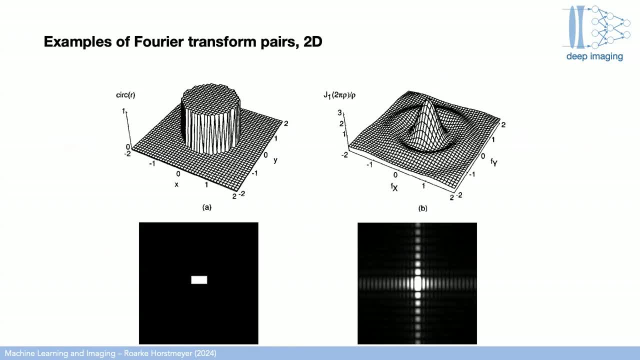 which is very common in imaging system analysis. It zeroes And then inside some circle, a defined radius, its value is 1. It kind of looks like the rect function: right Zeros and then ones inside. So, not surprisingly, it's very simple. 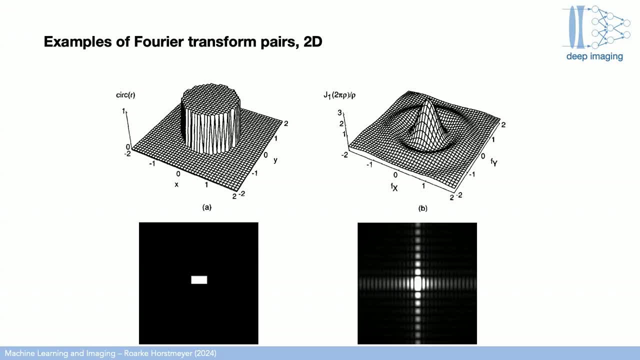 Fourier, transform kind of looks like a sinc function this way, but it's probably a jinx function. I don't know why, But it's similar. It's this whatever sinc-like function, It's just a vessel function. Here's a rectangle, a rect function. 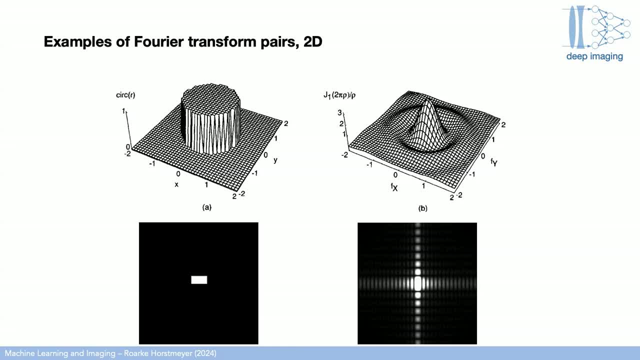 And it's Fourier transform. So the rect function is kind of a rect function in 1D. It's kind of replicated in the other dimension. So in this case the rect function is wider than it is tall, And so this property of Fourier transforms. 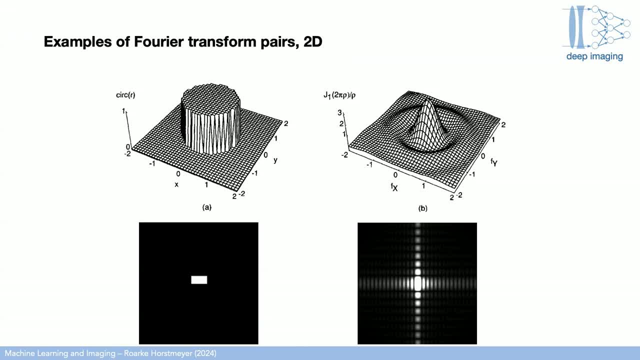 which hopefully we'll get comfortable with but might not be too new. If something you have a narrower function in one domain and you Fourier transform it, it's a wider function in the other right Narrow things become wide after a Fourier transform. 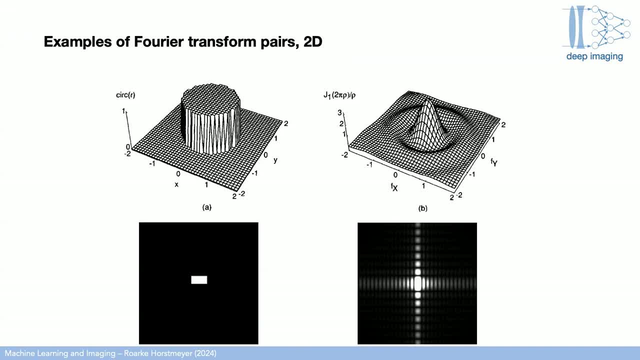 Wide things become narrow, And so the narrower part of this function becomes wider, And the wider part becomes narrower after this Fourier transform. So again, this is a separable scenario. This 2D function can be described by two separate 1D functions taking their outer product. 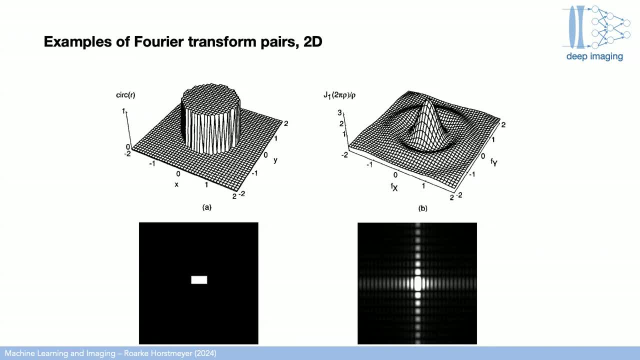 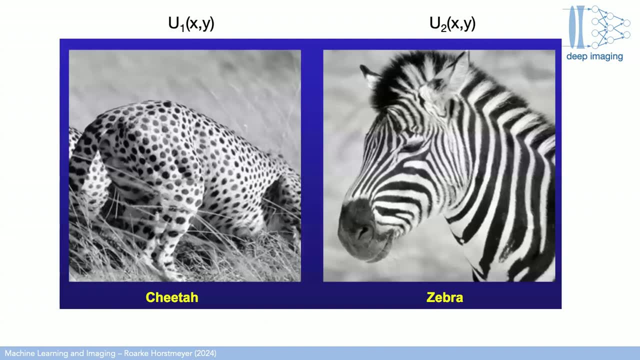 effectively. And so the same thing is true with the Fourier transform, And then you can take the Fourier transform, the 2D Fourier transform of any image really. And so here's- Here's a picture of a cheetah and a zebra. 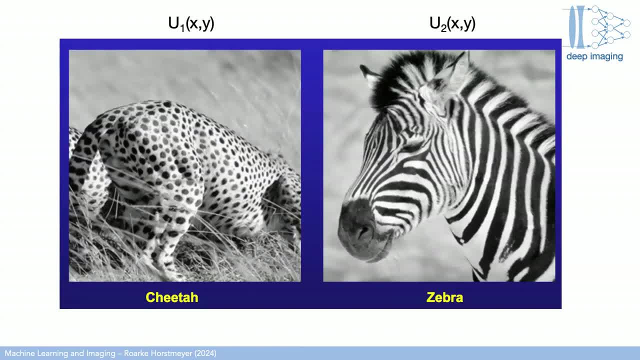 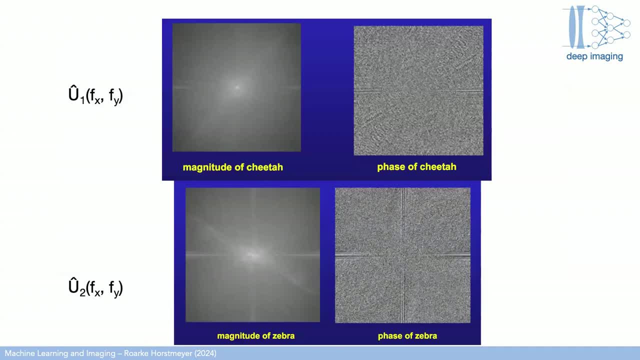 I just picked these at random because this is what popped up on Google, But here's their Fourier transforms, right And so importantly, just remember that Fourier transforms deal with complex numbers And so, generally, if you take the Fourier transform of something, and it is real and non-negative, 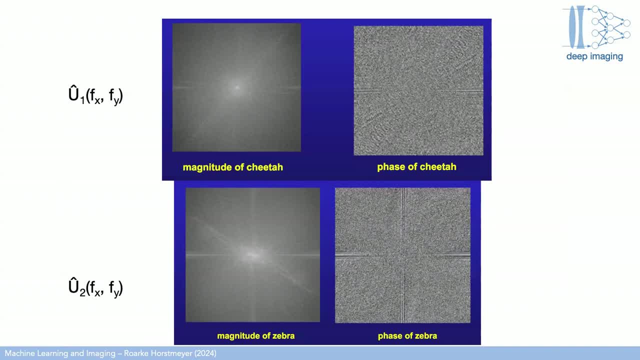 you'll end up with a complex function still, unless you're lucky in what you're taking. a Fourier transform of It's symmetric in two dimensions, which is very rare. So you have these weird distributions right, But all of these values describe the weight. 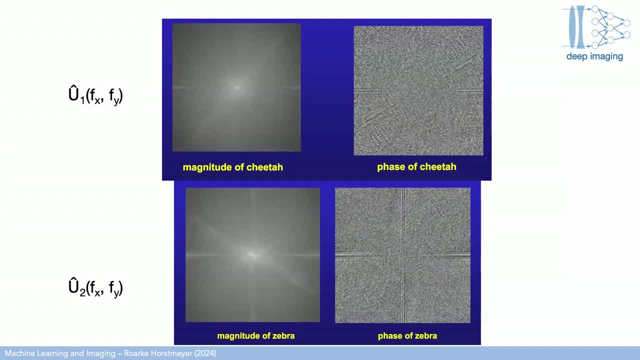 of different sinusoidal stripe patterns at different frequencies, to combine together to recreate that cheetah and the phase as well, And then here's the zebra, And so, yeah, you can kind of see there's these couple of things, couple lines in this cheetah image. 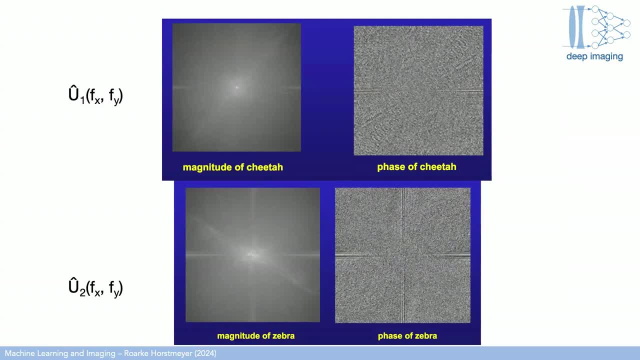 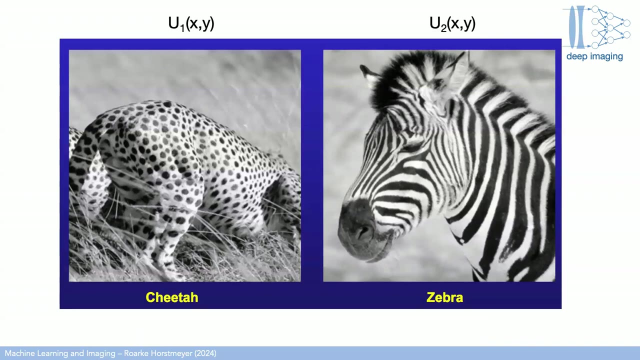 And then here there's a kind of diagonal line here in the zebra image. You look closely, definitely you can see it on the PDF versions, these stripes, And that's because here there's some particular stripes that are quite strong in the zebra right. 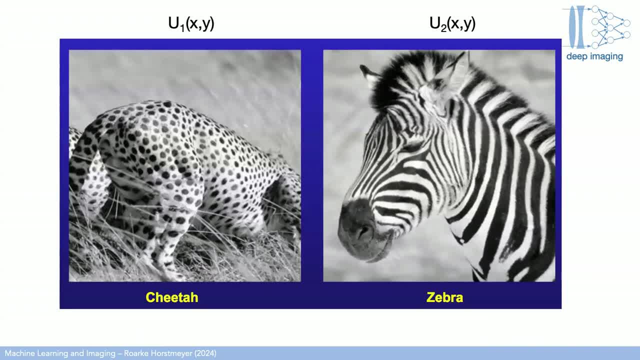 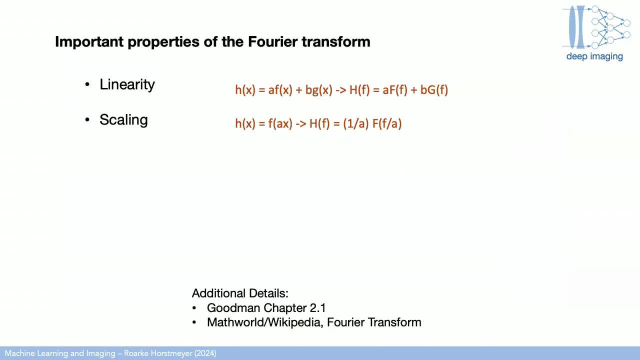 And then the cheetah. I think there's like kind of stripes hugged by the grass, And so that striping manifests itself in these larger values, in those particular diagonal areas of the Fourier transform. Fourier transform has all these nice properties too. It's a linear function. 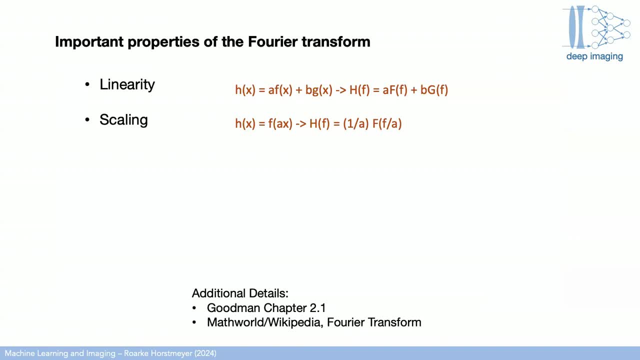 So, as the scaling and of course linearity Scaling, like I said, is a little bit unique in the Fourier transform, If you make something wider in one domain, it becomes narrower in the other right. So the Fourier transform has this inverse scaling property. 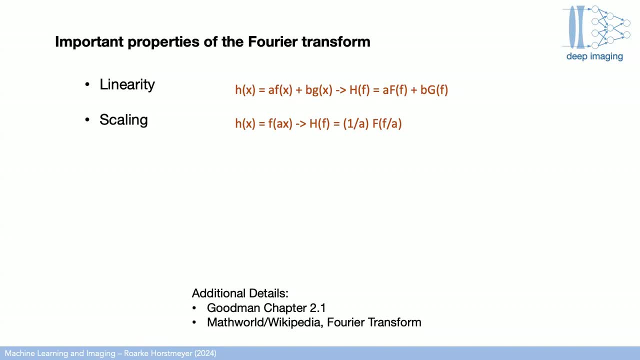 So if I make my rect function really wide, the associated sync function becomes really narrow, and vice versa. There's anyways there's other properties. I'm not gonna dwell on them. If you shift something, you pick up a phase ramp. 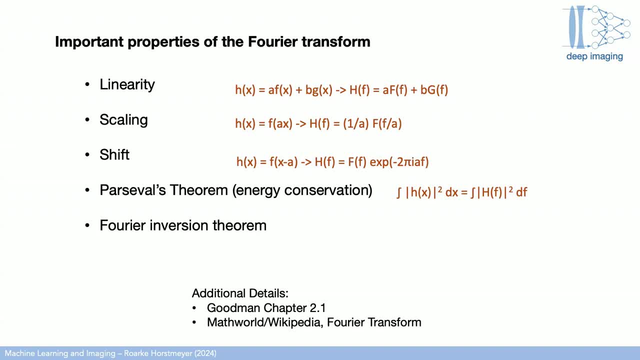 So this is an important theorem: The energy of a function and its Fourier transform are the same right. It's energy preserving which is physically useful, considering the application of Fourier transforms in our physical modeling. Okay, so this is the main thing I wanna impart. 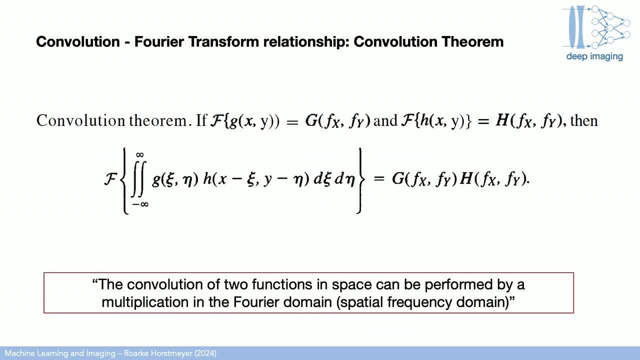 There's a convolution theorem, So it's always hard to verbally say this and it's also kind of confusing. It's confusing mathematically to write, And so we're gonna go through this a number of ways. I'll try to say it. 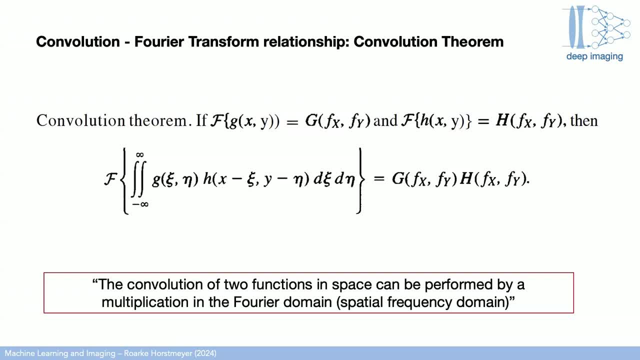 And I wrote it as simple as I could in this red box: The convolution of two functions in space or in general, can be performed by a multiplication in the Fourier domain. Okay, that's really what the simplest way to say this is. So if you wanna convolve two things, 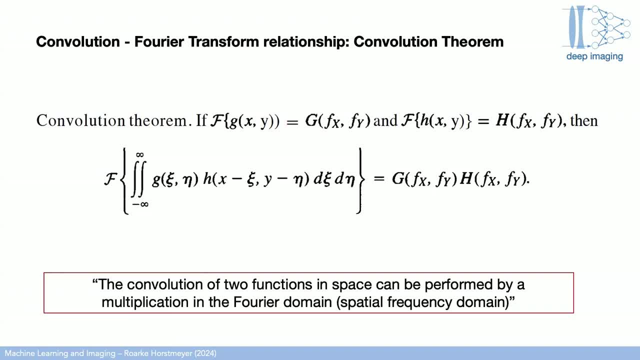 you wanna blur something, you can achieve it by doing Fourier transform, And so we'll start there. And so how Well, I'll explain in a second. But they're very analogous operations. What this equation says is that if I have a convolution, 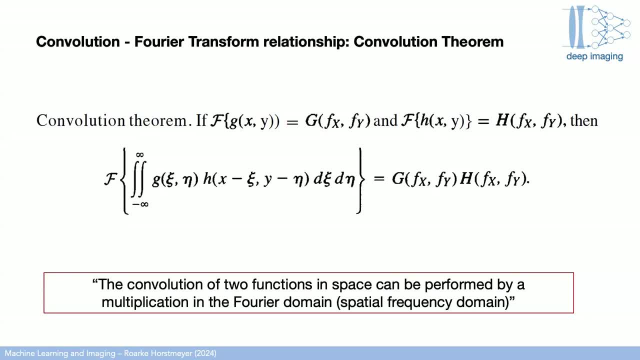 I blurred something. I had a input G and I blurred it. The output's the blurry result. I can take the Fourier transform of that blurred output. Okay, I can take it as my Fourier transform of the blurred output. We'll call that A, some quantity. 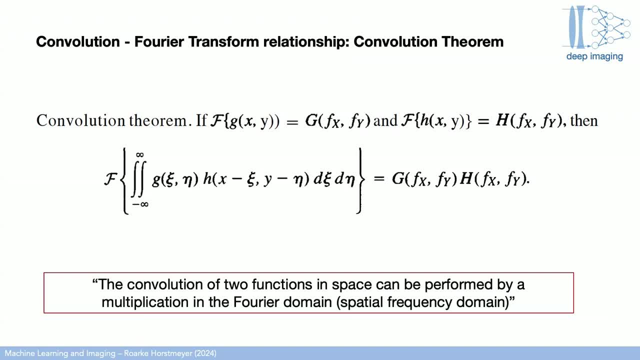 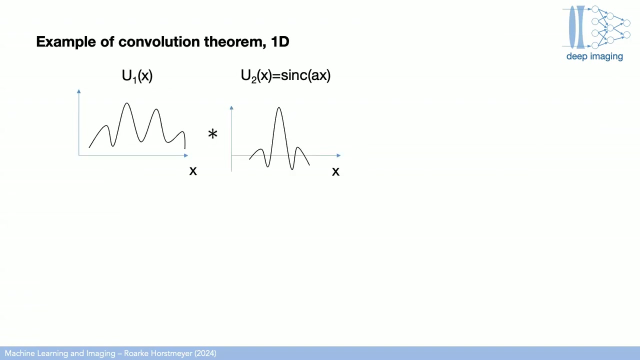 I can recreate that quantity by taking the Fourier transform of my input and the Fourier transform of my blur and multiplying them together. So I can do all my blurring just by taking two Fourier transforms and multiplying. Okay, So here's an example of that. 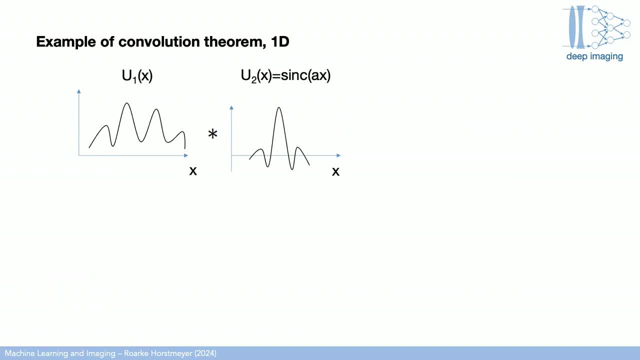 Hand drawn by me. We have a function and I do a convolution. I'm gonna use this symbol for convolution in this class. What I'm saying is I can take my input- U1, Fourier transform- And I can take my point spread function- U2 and Fourier transform. 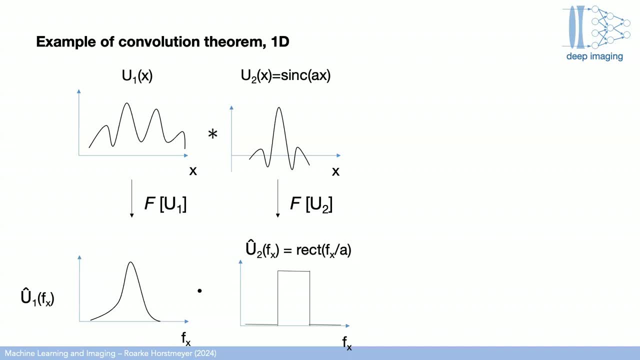 I drew a sink here, So this becomes a rect. So what I get is this kind of chopped off Fourier transform, right Cause this is gonna be a low pass filter. effectively, to my input, that's been Fourier transformed And what this convolution theorem says is I can take. 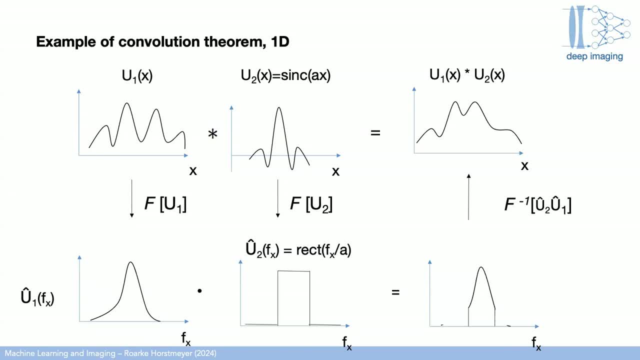 the this thing. I just created an inverse Fourier, transform and recover the convolution. So in my programming I can go along this top route, or in my math that I'm doing, writing all these convolution operations down and equations to solve them. I can stay up here and you'll be fine. 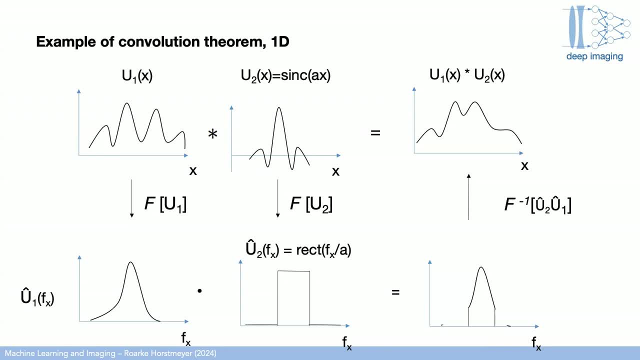 but it's pretty tedious to do that. It also gets computationally expensive to do that, And so a computationally more efficient way to achieve this is to use the Fourier transform, And also sometimes intuitively helpful way to think about this is to go this bottom route. 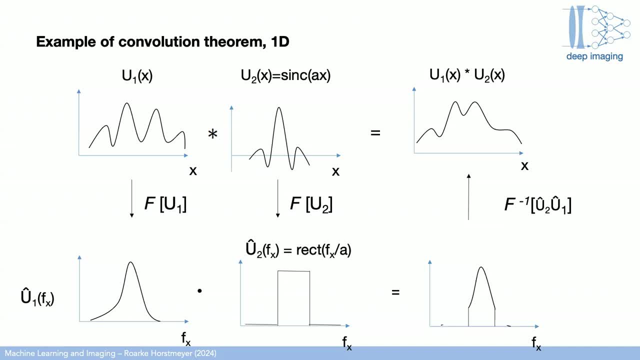 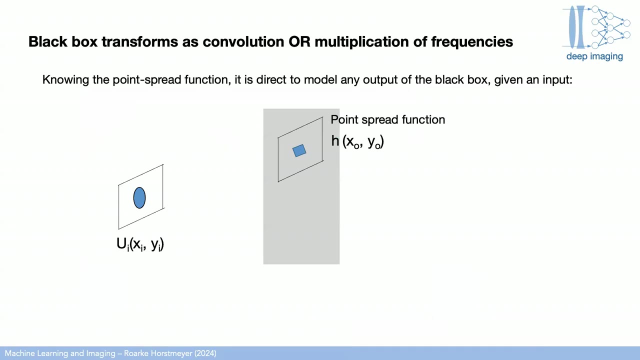 And you take the Fourier transform, take the other one, multiply them. You end up down here and then you can always jump back up with an inverse Fourier transform. All right, So in this picture we have this input in 2D and a point spread function H. 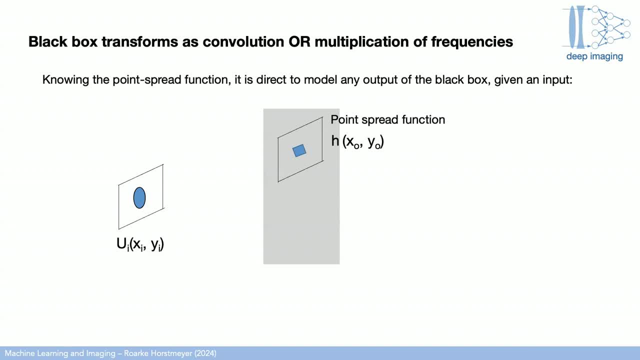 What I was saying before is all we need to know is this point spread function H to know the impact or the effect of this black box transformation. Not surprisingly, I can also say: well, instead of knowing this point spread function H, I can just know it's Fourier transform, right. 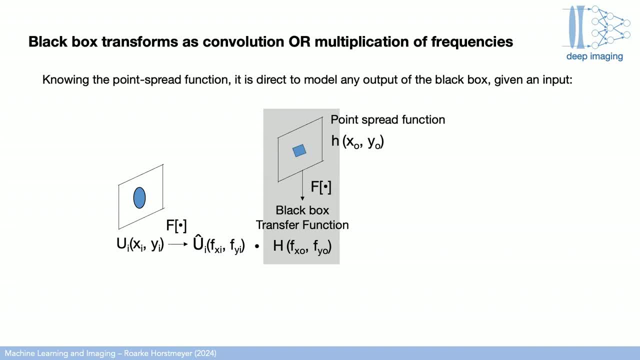 And that's this big capital H. So that capital H is called a transfer function. You've probably heard of it. It's incredibly useful in the analysis of circuits, right, And even audio signals and all that sort of thing. But here we're talking about it in terms of an imaging system.